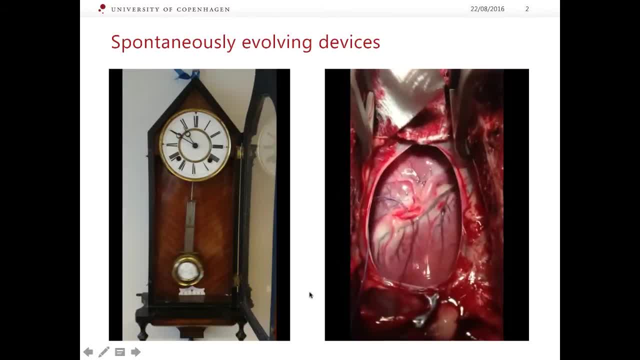 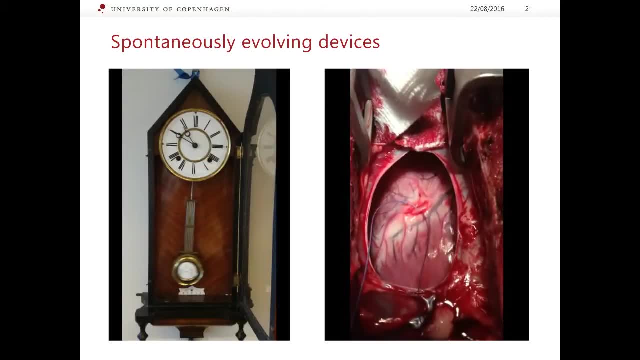 Now take a biological system, For example. this is the heart of a man-made device. When it is properly wound, the pendulum is swinging all by itself. over 50 kg. Danish landrace pig. While sitting inside the body, the heart beats spontaneously. 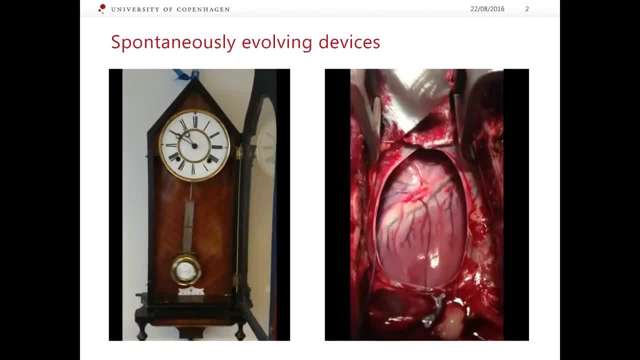 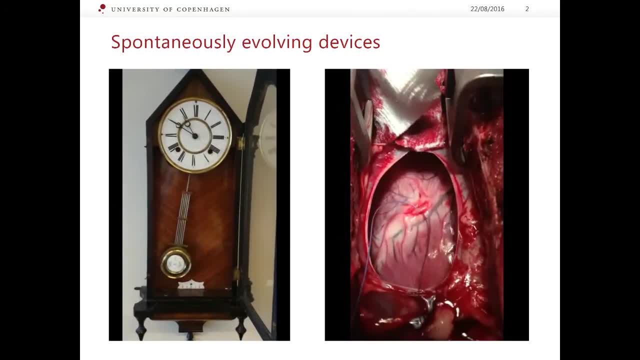 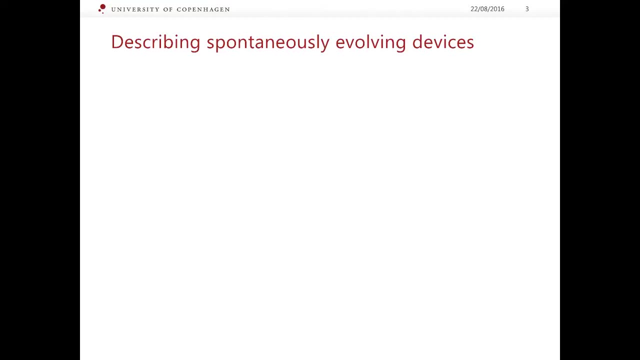 and again, no external manipulator dictates the heart when to contract next. This applies to all hearts of all animals. To describe spontaneously evolving devices mathematically, we need certain mathematical tools If we make an assumption that our devices or organs evolve in continuous time and 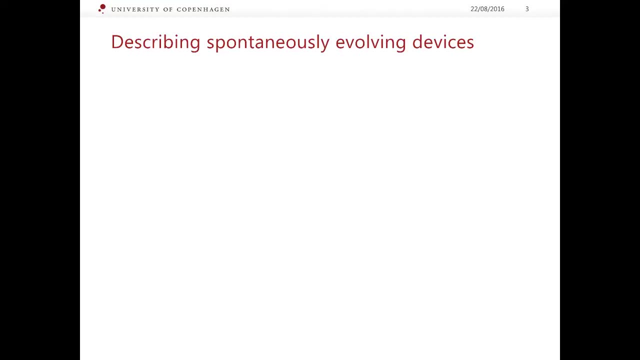 if we assume that their states are changing continuously, then their suitable models will typically take the form of ordinary differential equations. Of that form, an abbreviation is ODE. An ODE is described as a function, capital F, whose arguments are time, t, x, the variable that changes with. 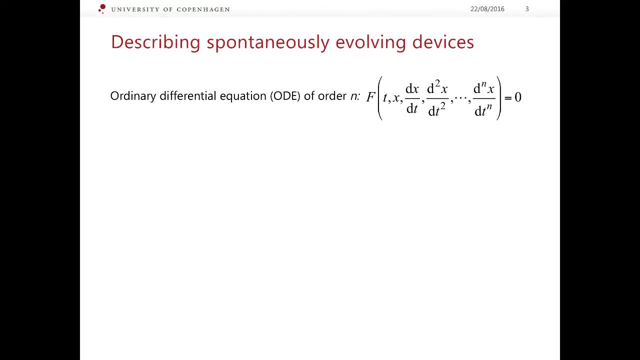 time and several of the time derivatives of this variable, And this function is typically equated to zero. It is convenient to introduce the following notation: Instead of writing dx by dt each time, it is convenient to write x, dot, and we use dots up to the time. 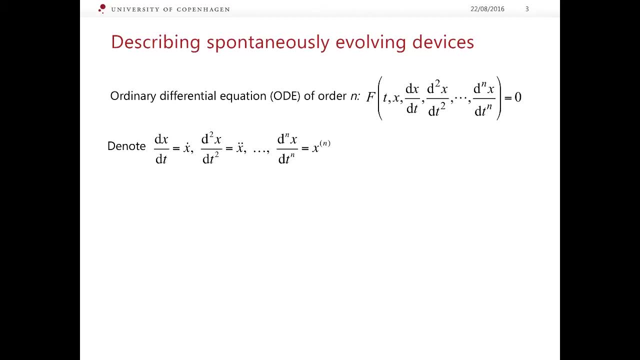 derivatives up to the third order, For time derivatives of nth order. when n is greater than 3, we write the order n inside the brackets and put it in the superscript of variable x. Now the general ordinary differential equation of order n can be rewritten as follows: 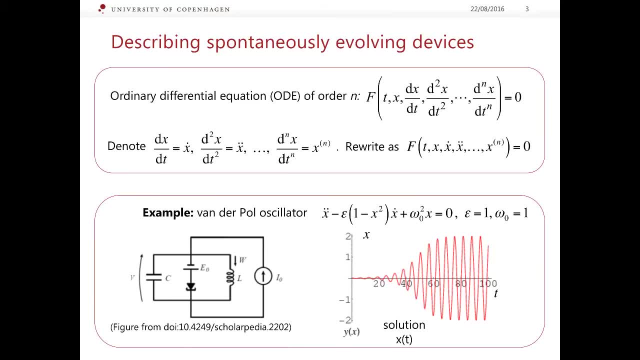 A very nice example of such an ODE is a famous Van de Pol oscillator which describes the behavior of voltage in a certain electronic circuit whose sketch is given by one-dness radius. And we have a basis for this equation, In that case for us. 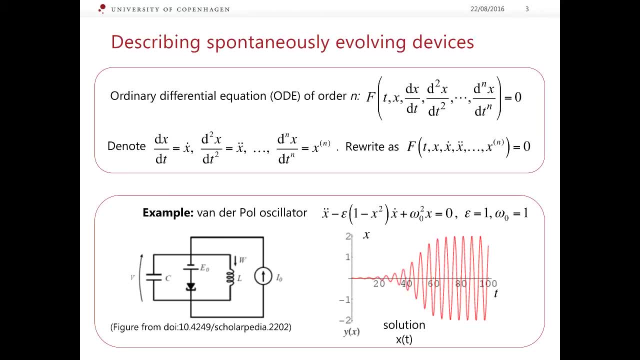 is given in the left-hand side of this figure. Variable x is the unknown variable, which is equivalent to voltage. after the change of variables. You can immediately see that this equation is nonlinear because of the term x squared multiplied by x dot. Here, epsilon and omega zero are some parameters In the right-hand side of this slide. 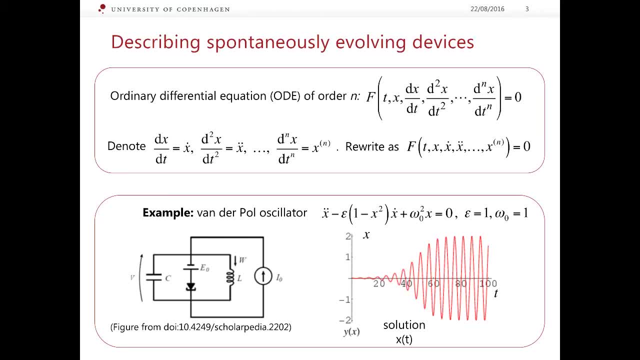 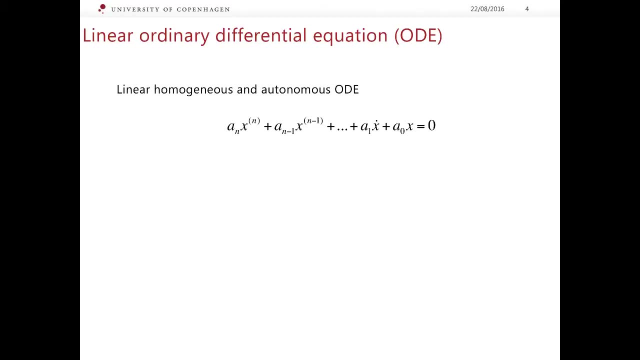 a red line shows the solution of this equation obtained numerically. Let us consider a simpler version of ordinary differential equation And, in particular, let us consider an ODE which is linear, homogeneous and autonomous. This equation has the form shown in the slide. 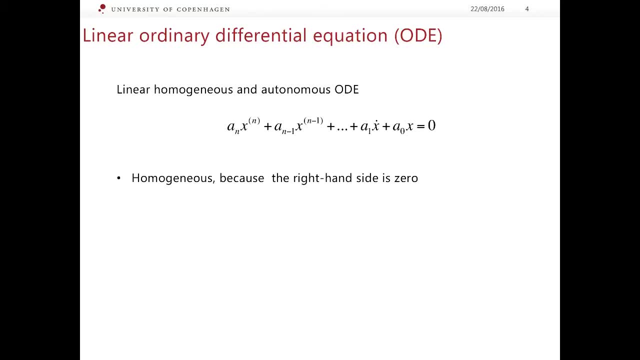 This equation is homogeneous because the right-hand side of this equation is identically equal to zero. and this equation is autonomous because the coefficients a, n, a n minus 1, and throughout to a 1 and a 0 are all constants, which means they do not depend on time. 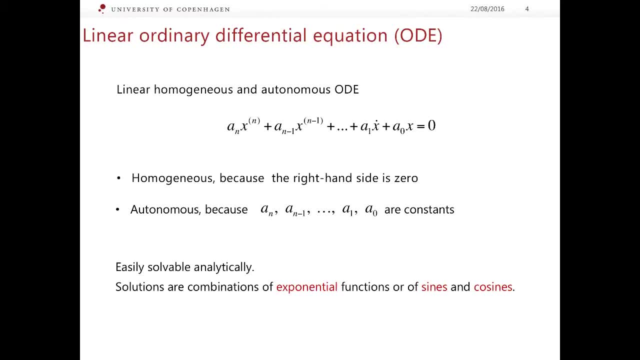 Equations of this form can be solved analytically exactly and quite easily, and their solutions can be represented as combinations of certain exponential functions or combinations of sines and cosines. Consider an example of such an equation, and this example describes small. 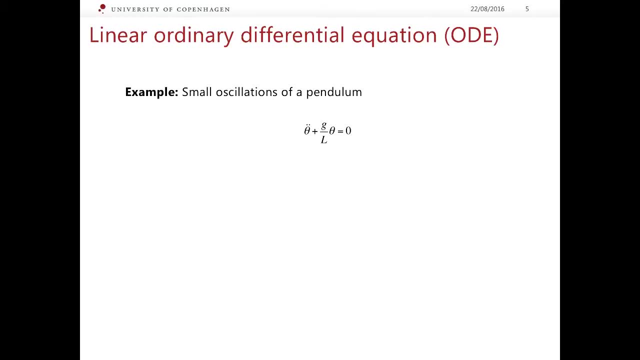 oscillations of a mechanical pendulum. This equation is an equation for the angle the pendulum makes with the vertical, So this angle, theta, is evolving with time. The solution to this equation is represented here as a sinusoidal function of time And the frequency. the angular frequency of this sine is equal to the square root of the factor. 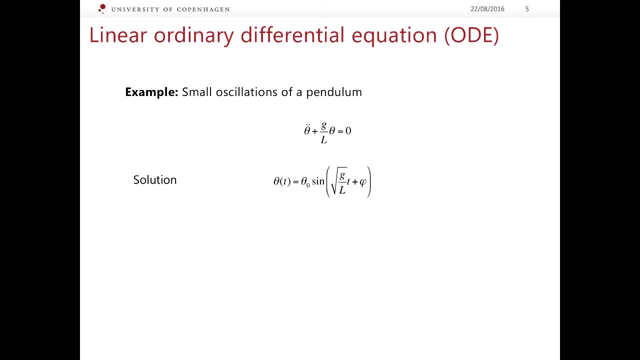 g over l in the ODE phi is some initial phase shift and theta0 can be found from initial conditions. Please note that even linear ordinary differential equations which are non-homogeneous and or which have coefficients depending on time might not be solvable with that ease as the 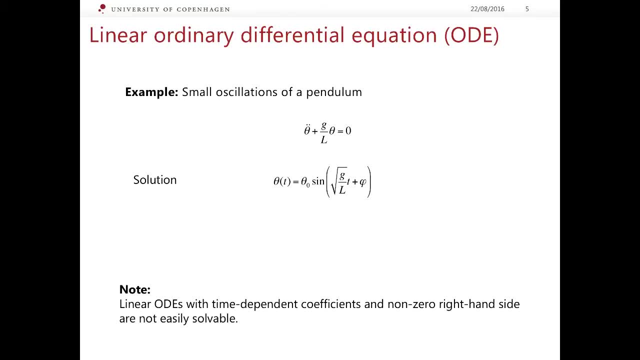 equation which we considered just now. What about more complex equations? In practice, realistic models of real devices or organs have the following feature: They are non-linear. They must be non-linear if they need to be realistic, Which means that their models should be represented by some non-linear ODE. 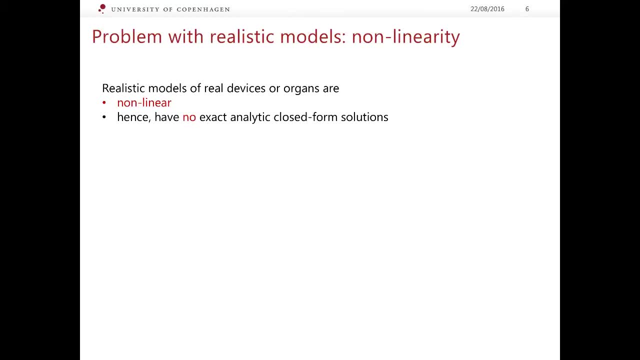 And such non-linear ordinary differential equations unfortunately very rarely have exact analytic solutions in the closed form, Almost never. Look at the same example Van der Pol equation describing an electronic circuit. Well, this is obviously a non-linear equation, Okay. 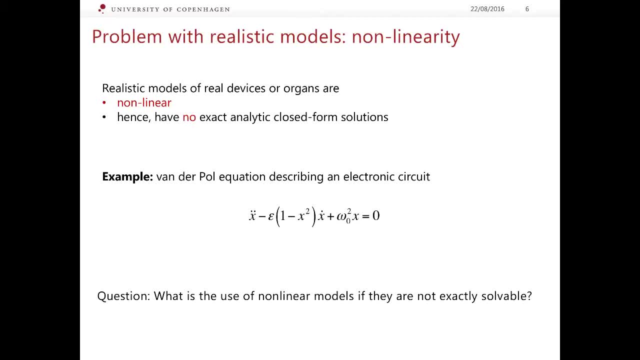 It can be solvable only numerically. And let us ask a question which is very pertinent here: If realistic models of real devices or organs cannot be solved analytically, and exactly what's the point even writing down these models? Are they completely useless? 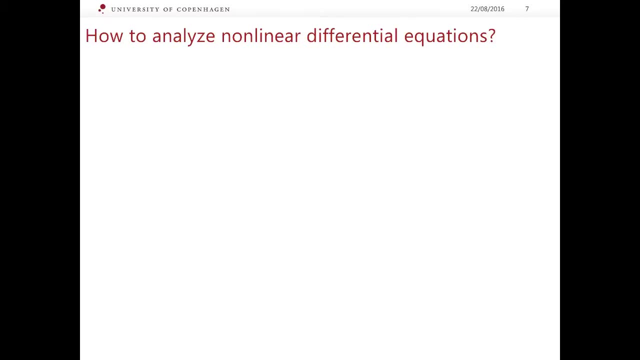 Fortunately, the situation is not quite hopeless as it might seem. We will consider three general approaches to deal with non-linear differential equations. The first approach is kind of obvious- is to solve this equation numerically. An advantage of this approach is that if the solution to the ODE exists in principle, 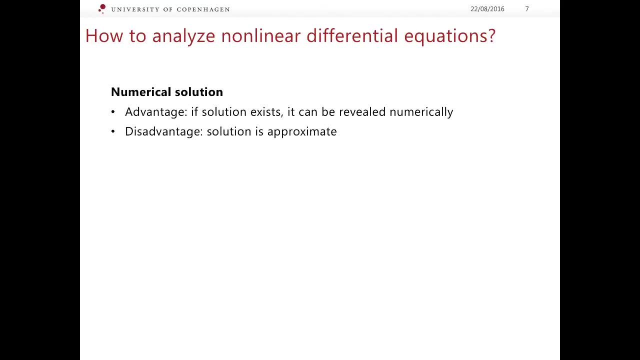 then, numerically, it can be revealed, And the disadvantage is that, unfortunately, numerical solutions can only be approximate. They will never be exact. The second approach concerns geometrical methods, and it is thanks to the great breakthrough which occurred in the 19th century, mostly thanks to a great mathematician, Henri Pornkelder. 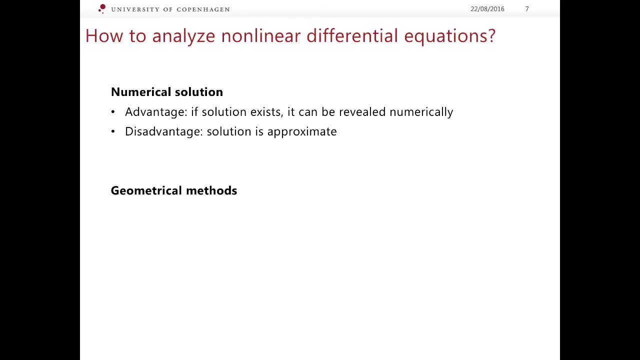 Poincaré. Poincaré proposed to represent solutions of ordinary differential equations as certain trajectories, geometric sets in certain spaces, which are called phase spaces. This way, if the solution is a geometrical object, we can consider the behavior of a nonlinear ordinary differential equation using 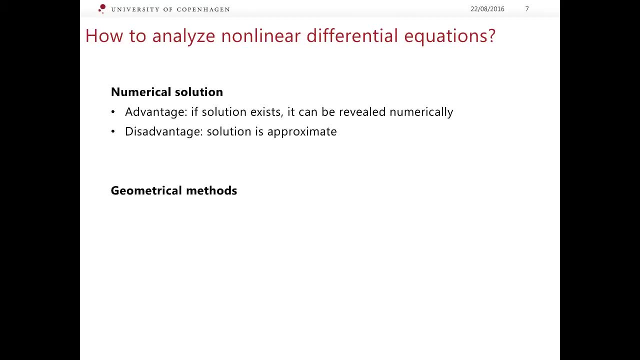 some geometrical approaches which rely a lot on visualization and on some visual information. The advantage of such methods is that the properties of solutions can be revealed at a qualitative level at least However. However, there is a disadvantage that such methods require some form of visualization. 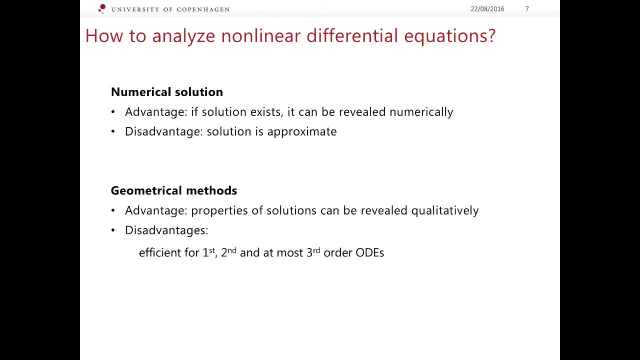 or imagination in a space whose dimension can be 1,, 2 and, at most, 3.. Unfortunately, when this space has larger dimension, which will be the case for higher order non-linear differential equations, this approach is not quite efficient Because we cannot visualize such solutions. 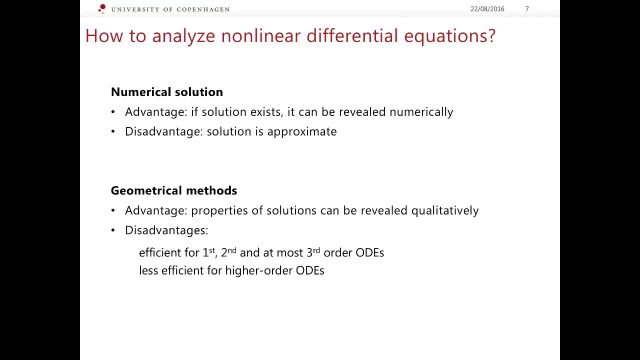 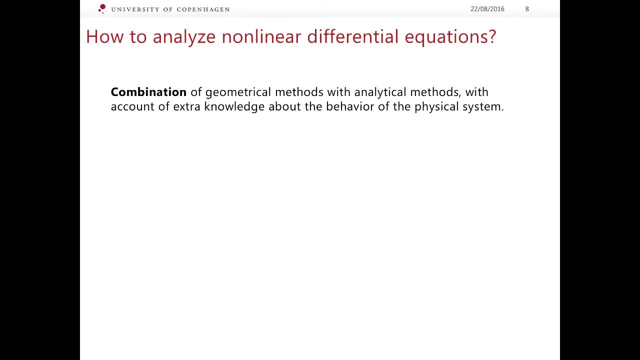 So for higher order ODEs this approach might not be quite appealing. And there is a third approach which combines the geometrical methods with some analytical tools and with some knowledge about the behavior of the physical prototype of our equations which is available typically. 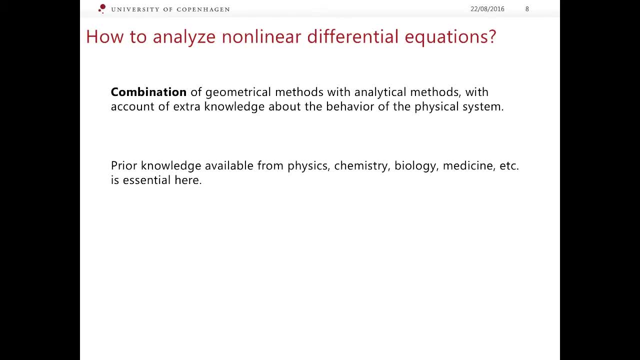 So let's take a look. It is essential here that such an approach really requires additional knowledge in physics, chemistry, biology, medicine and maybe in some other related disciplines. Without this knowledge, it might be really difficult to make any specific assumptions regarding the properties of solutions of our differential equations. 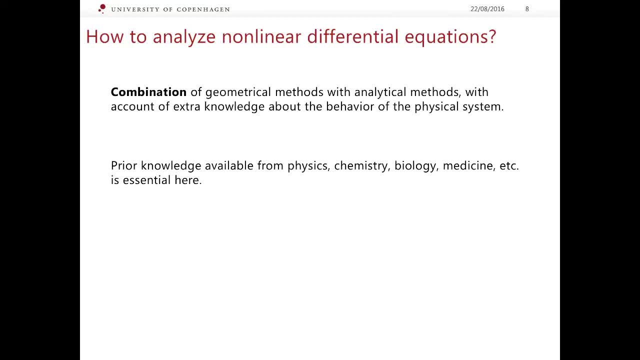 And there is another approach which also requires a multi-disciplinarity. All the three approaches considered here require introduction of a certain mathematical concept called a dynamical system. A dynamical system has two components. We will consider autonomous dynamical systems in the first instance. 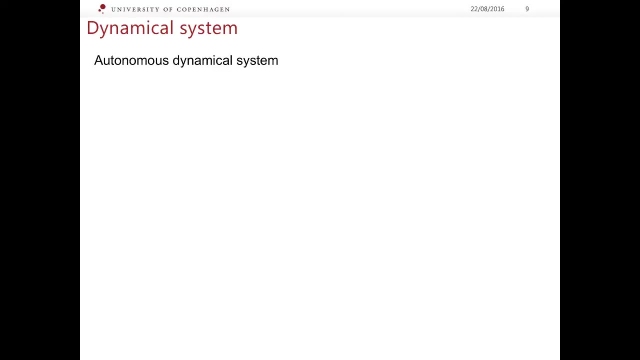 The first component is not a dynamic system. It is a form of composing. So our dynamical system is constituted by değişująщее. The second component is called an autonomous dynamical system. The third component is a dynamic system. The first component of a dynamical system is the phase space. 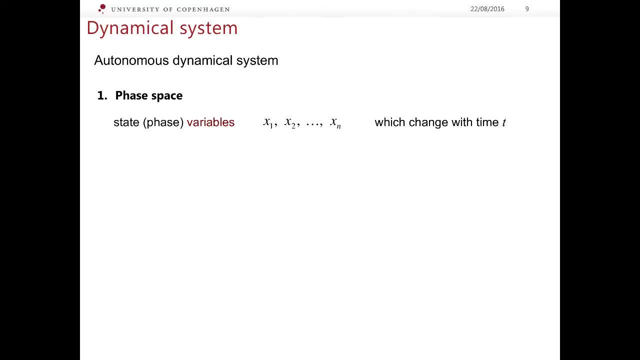 To introduce the phase space, we need to identify some quantities which change with time. These quantities are called variables, or more precisely, state variables, and their number should be sufficient to describe the state of the system at any time, moment t. Now let us introduce the following coordinate axes for all the state variables involved: 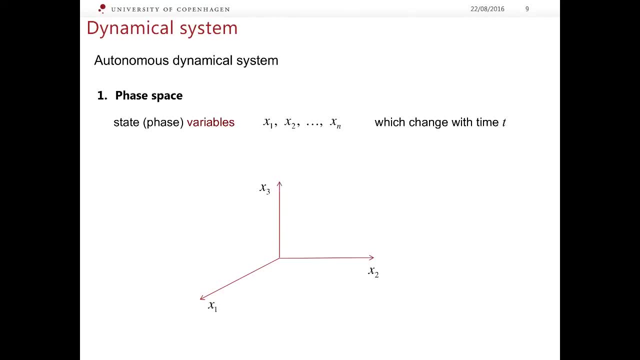 x1,, x2,, x3, and we can continue to xn. Let us construct a vector from the state variables of this system. The vector is denoted as a thick letter x. Every state vector is represented as a single point in this space, and because all variables 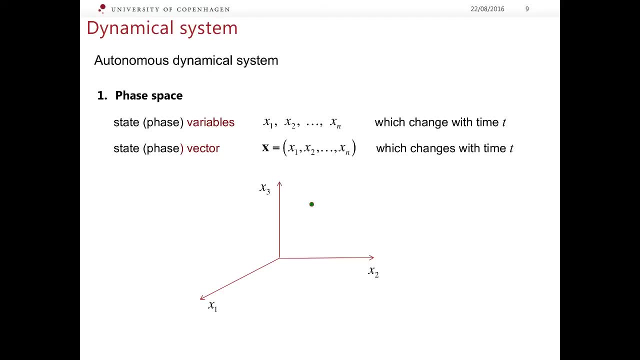 will change with time. the vector x will change in time too, which means its representative point will change Like this. So let us start Now. we can introduce the phase space as the space of all possible states of the given system. The second component of a dynamical system is evolution operator. 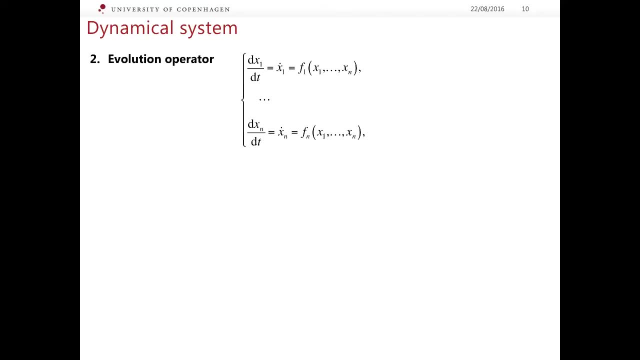 What is it about If we represent the dynamical system in the following form? it means that we write the state and the number of points representing it. 2. For each of the paths we introduce a different variant of the system. The time of the time when the process of evolution gets to a certain point depends on the state. 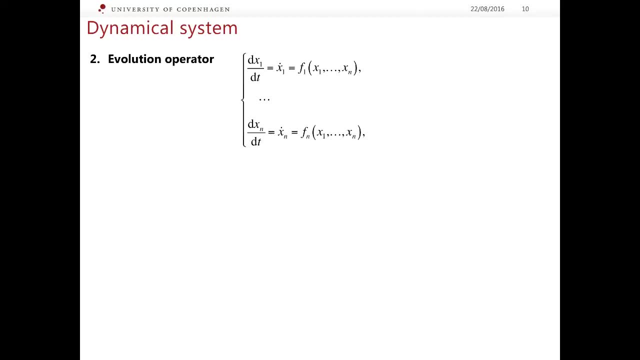 of the system. Let us start, So let us write down n equations which are, first order, ordinary differential equations. Each equation corresponds to the phase variables introduced on the previous slide. For each variable, we introduce the quantity, the rate of change of this variable, which. 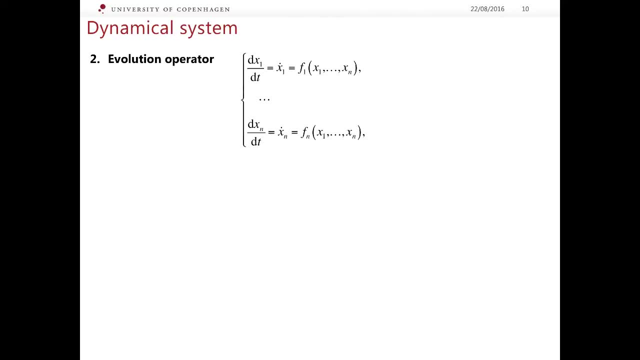 depends on the current state of the system. 3. The same system can be rewritten in a more compact vector notation as shown here. Now consider the phase space of this dynamical system. For simplicity we show a three-dimensional space And of course every state is represented as a single point. but it is convenient to 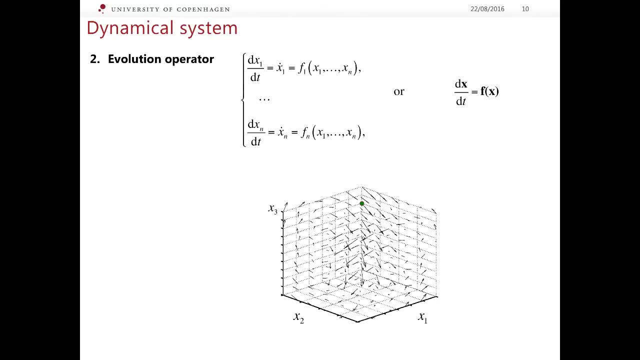 introduce a special vector whose components are formed by the values of functions f1, f2, etc. up to fn, which take certain values at the given state. This set of functions form a vector which is shown by green in this slide. 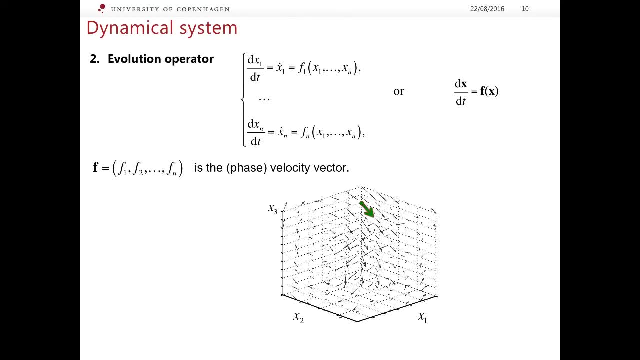 This is called the phase velocity, And the phase velocity vector is shown by green in this slide. As time goes by, the state of the system changes and the velocity vectors are generally different for different states. The full collection of the velocity vectors corresponding to all possible states is: 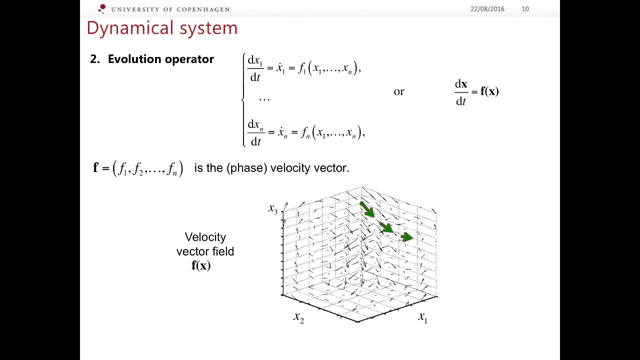 a kind of linear feed. It is important to note that each field contains a function f1 that corresponds only to a velocity vector field and the untrans compilation of the velocity vector field contains a�f1.. 1I manage two time zones. 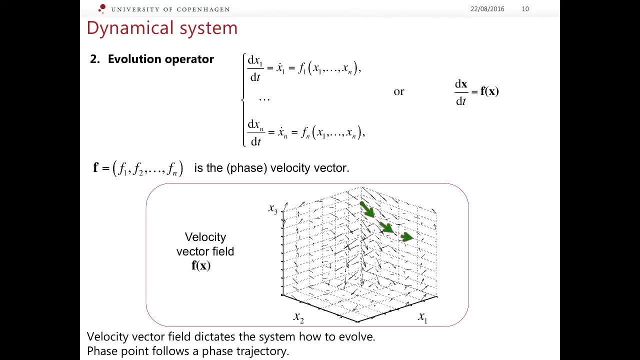 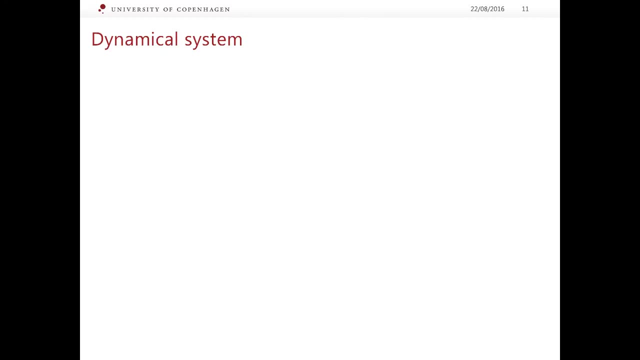 I AG Above and below the phase category: delta, Forowser B and V BW- See here. pulsiv vectors will be tangent or they will be touching the phase trajectory at each point. Let us consider an example. It is the same Van der Pol oscillator as we considered before, but here I rename the quantity. 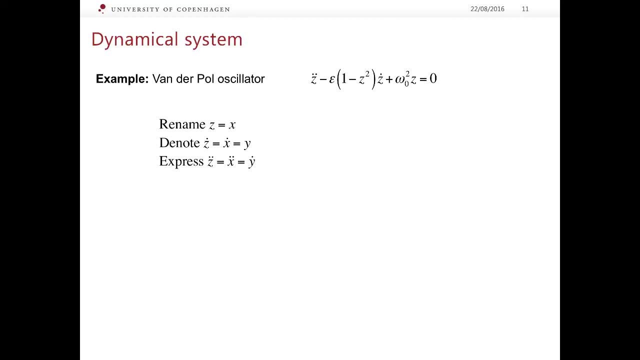 x by the quantity z, for convenience, Now do the following: We now rename z as x and we introduce a new variable, y, which will be the first time derivative of the quantity z, which is the same as the first time derivative of the quantity x. 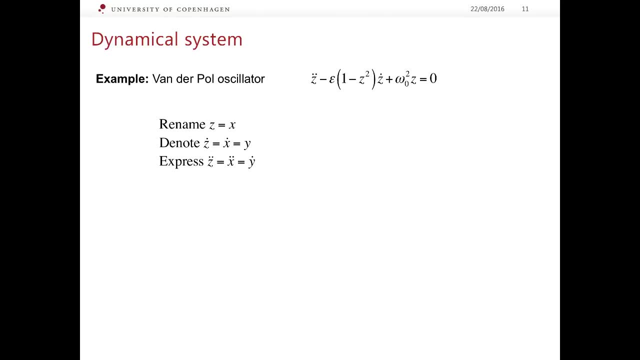 And now we can express the second time derivative of z as the first derivative of y. This way we effectively introduced two state variables, x and y. And now we can express the second time derivative of z as the first derivative of y And we can write down the system above the ordinary differential, above as a system of: 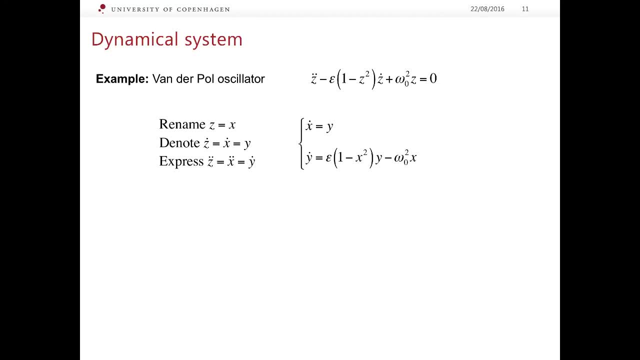 two first-order ordinary differential equations which in fact define the dynamical system. Let us denote the right-hand sides of this equations as f1 and f2.. The figure shows the phase space of the given system which goes right to which works the 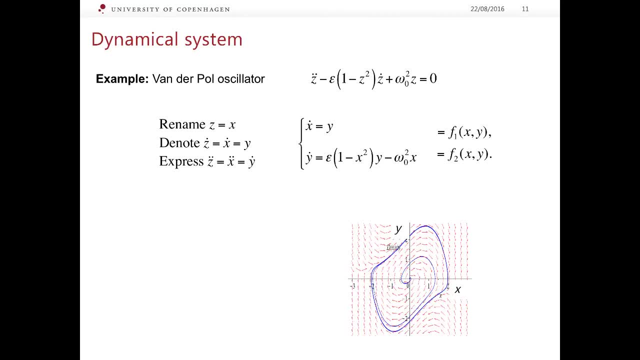 dynamic line and this is going to be the differential Superman. pressure spreads and now you see a dimension where the value of the voltage changes. Since the Frauenstein equation, in fact, is the facet of this. differential laws in fact, appears to be the phase plane, because the dimension of this system is 2.. 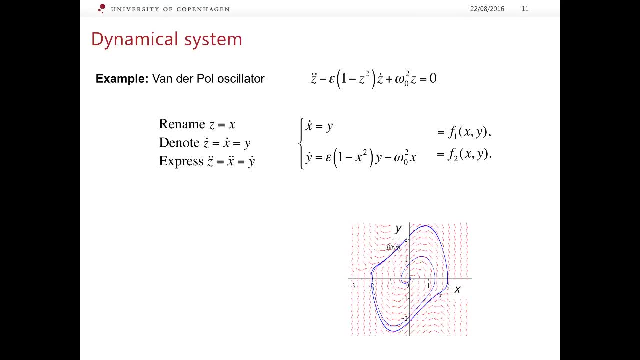 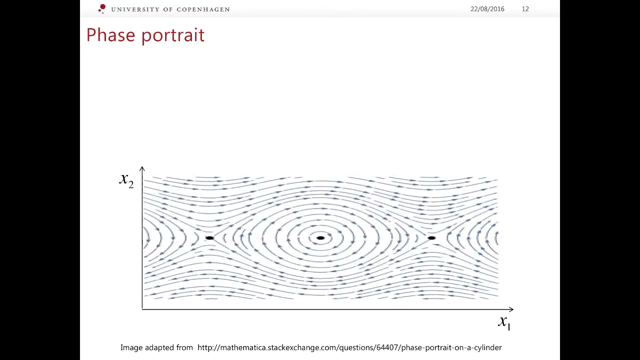 x and y are our state variables, Red arrows show the velocity vectors- and one of such vectors is shown here- And the blue line shows the phase trajectory which follows the instructions obtained from the velocity vector field. Let us now introduce a very convenient concept of a phase portrait.